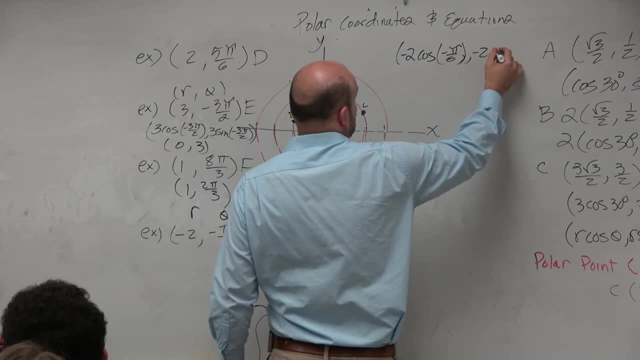 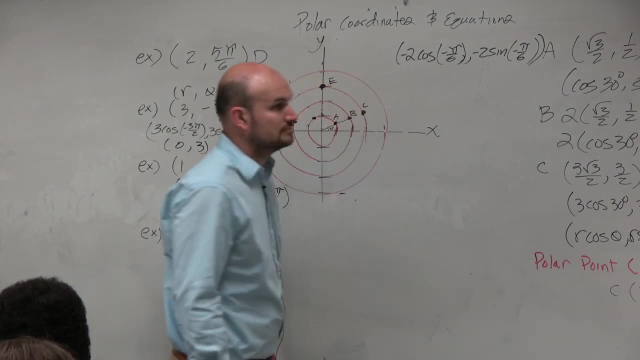 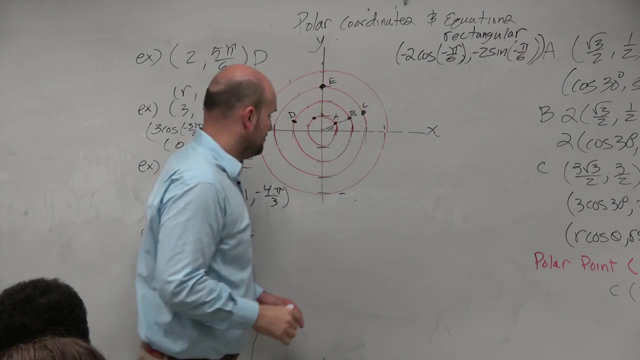 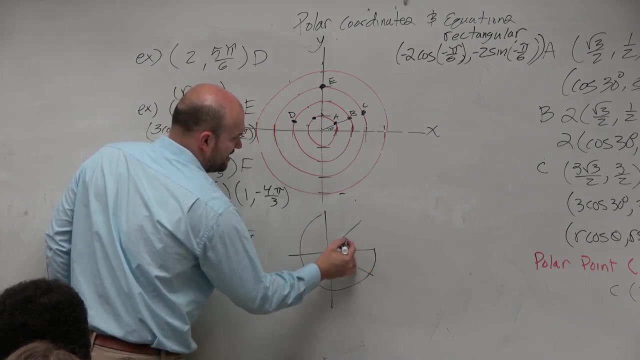 and comma negative 2 sine of negative pi over 6.. Everybody else? okay, That's the rectangular form, All right, Based on our unit circle. do we remember what the coordinate point is for negative pi over 6?? So over here is pi over 6.. 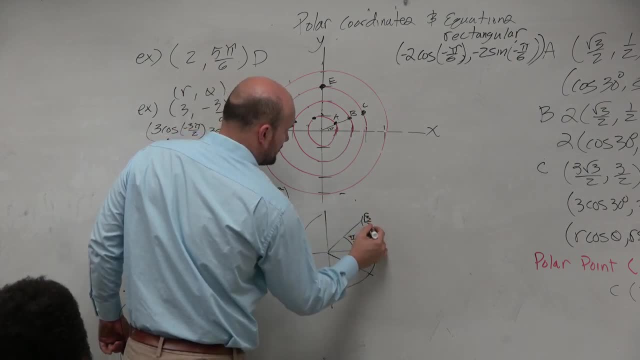 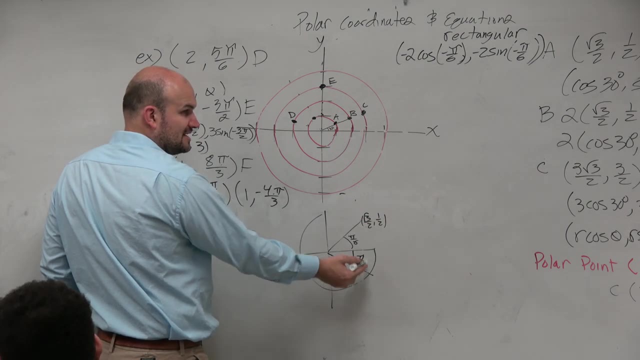 They have the same reference angle. This one is square root of 3 over 2 comma 1 half. So if I have the same reference angle but it's in the negative direction, I'm basically just reflecting this point across the x-axis. 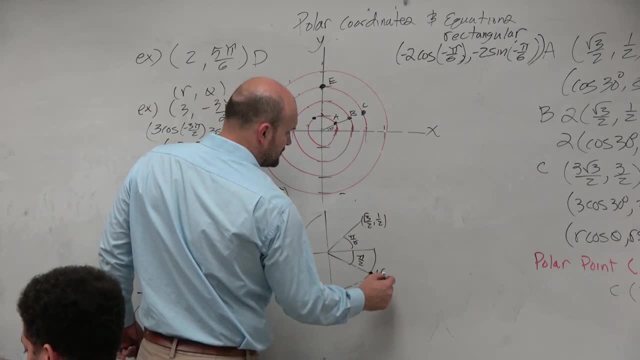 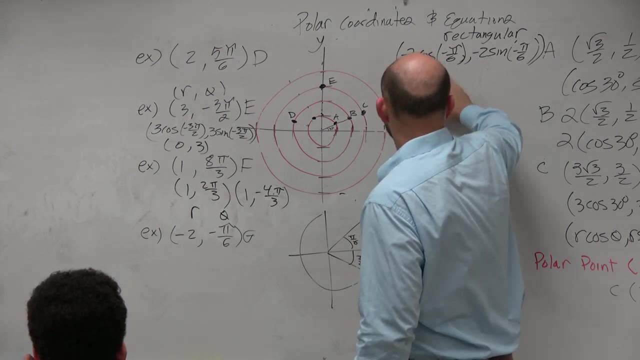 So, therefore, what's going to happen? What's going to be? negative The 1 half, So I have square root of 3 over 2 comma, negative 1 half, So really I'm doing negative 2 times cosine of negative pi over 6,. 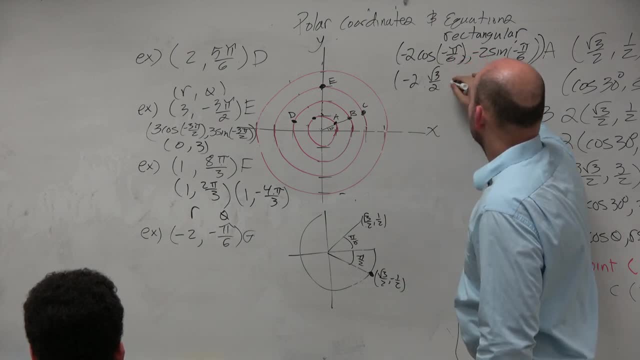 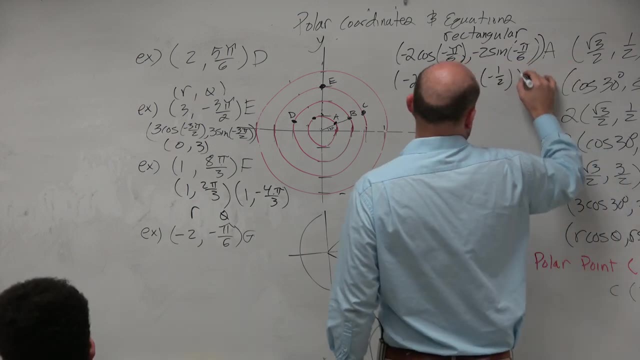 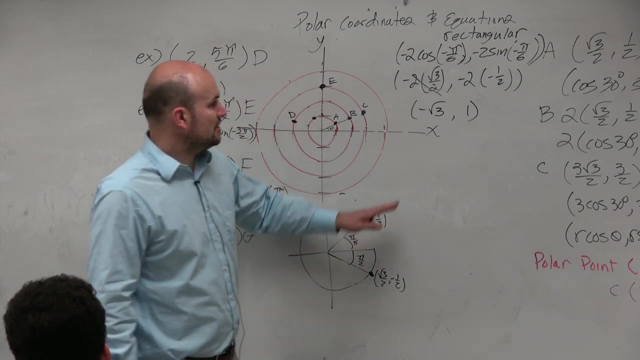 which is square root of 3, over 2, comma negative 2 times sine, which is negative 1 half. So therefore I get negative square root of 3 comma, positive 1.. So let's graph This point. 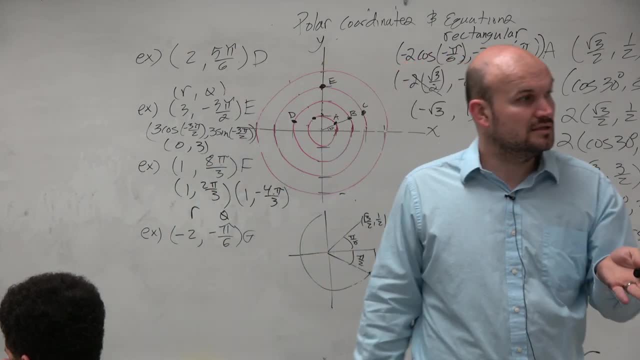 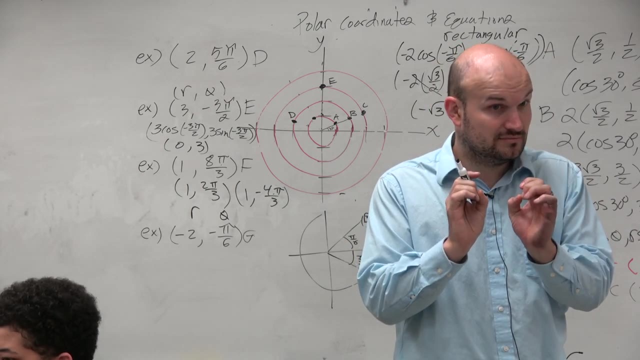 So let's think about this: Square root of 4 is 2.. Square root of 1 is 1.. So the square root of 3 should be somewhere in between 1 and 2.. Like one point. 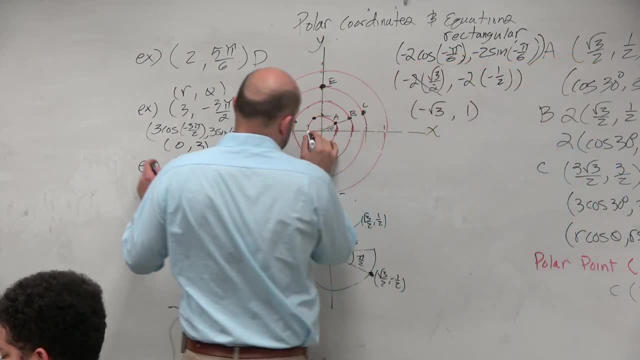 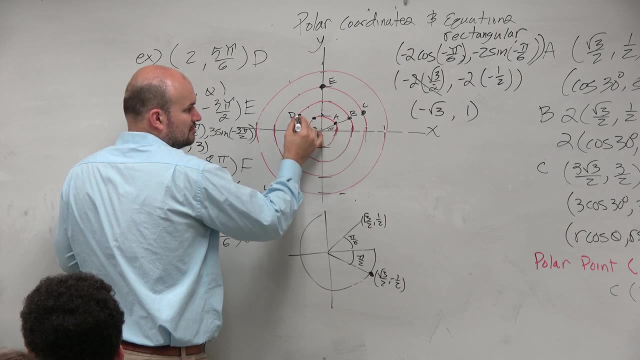 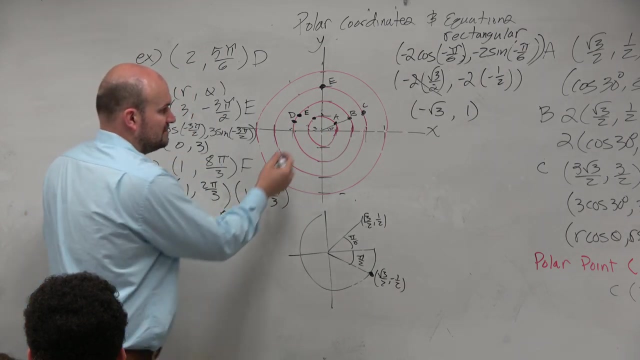 I don't know Something. So this is roughly somewhere between negative 1 and 2.. This point is 1.. So does it look like that point is right there, kind of Like roughly? Does that make sense? Here it's at 1, right. 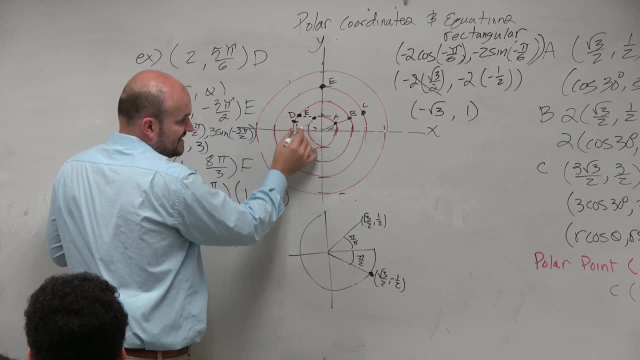 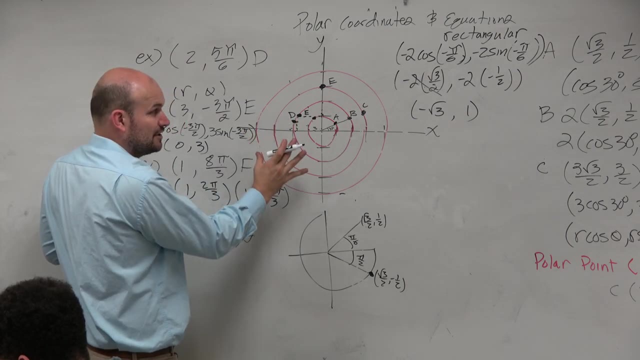 The height is 1.. And then this point is somewhere some decimal between 1 and 2.. I don't know what it is, I'm just estimating, right, Just estimating the decimal, But that relatively makes sense. Rectangular. 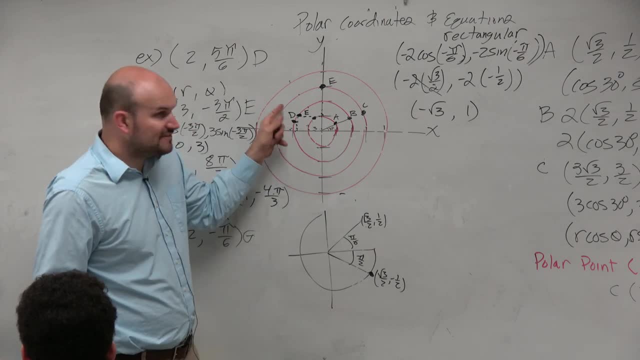 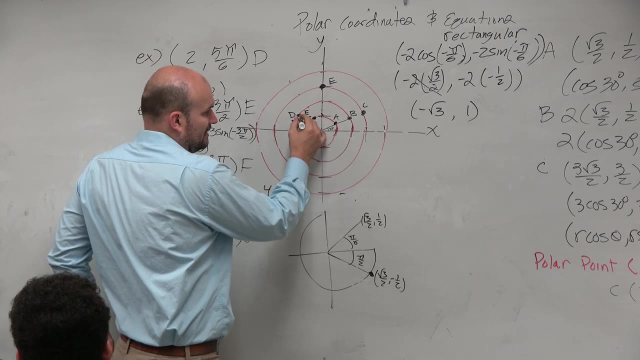 Now, if we look at this polar, we need to represent this polar. We have the same radius, which is 2.. Now we've got to think about, though: what should our angle be? Or is our angle? Now, let's think about a rectangular form. 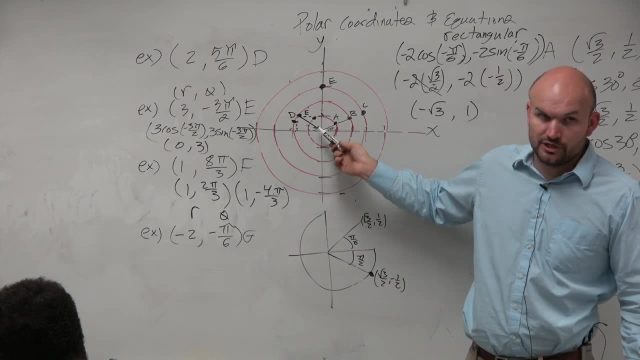 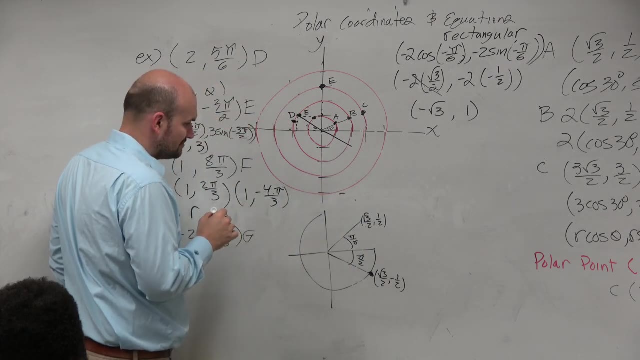 OK, Is that angle negative pi over 6?? Like no, That's not. Obviously that's not negative. Negative pi over 6 is over here, right? Is that supposed to be pi over 2? No, it's supposed to be 6.. 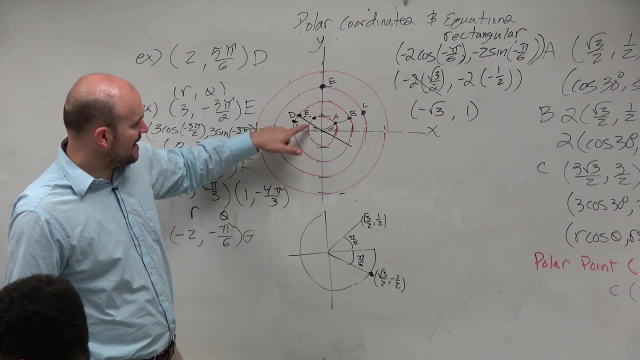 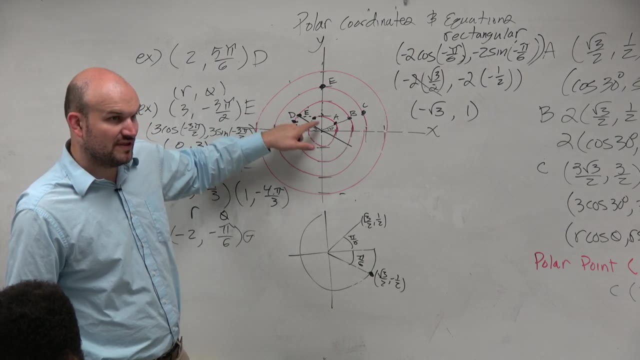 But negative pi over 6 is like over here. But do these angles like I'm just drawing from 0,, 0 to that coordinate point And then I'm drawing like negative pi over 6. Don't these angles kind of look like pretty close, like reflections of each other? 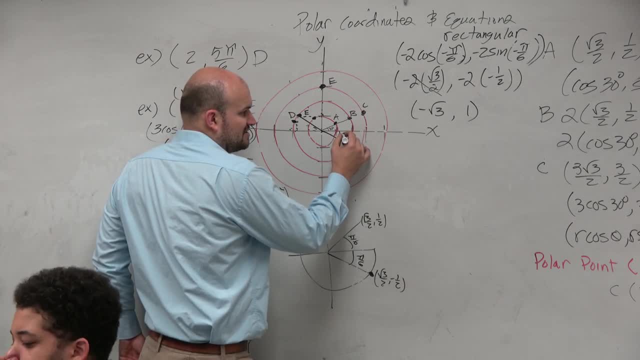 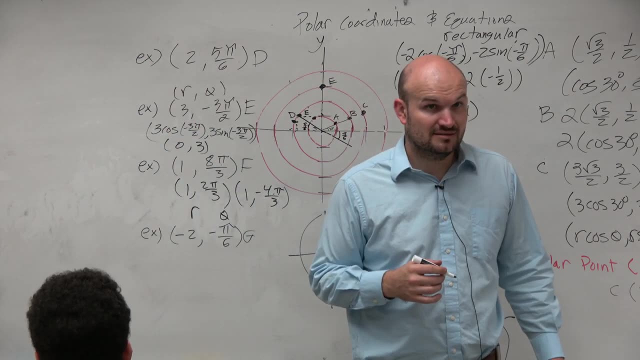 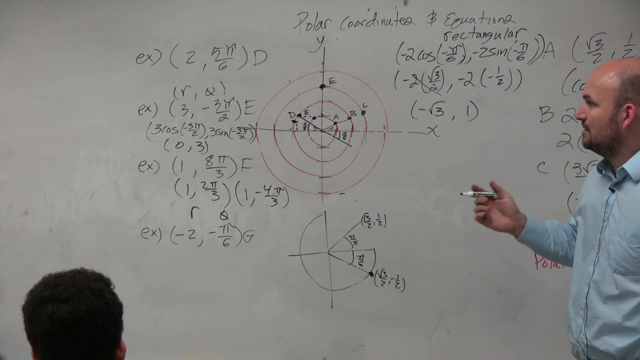 Like where almost I can basically assume that If this has a reference angle of pi over 6, then this has to have a reference angle of pi over 6? Yeah, So basically there's well, first of all my coordinate. 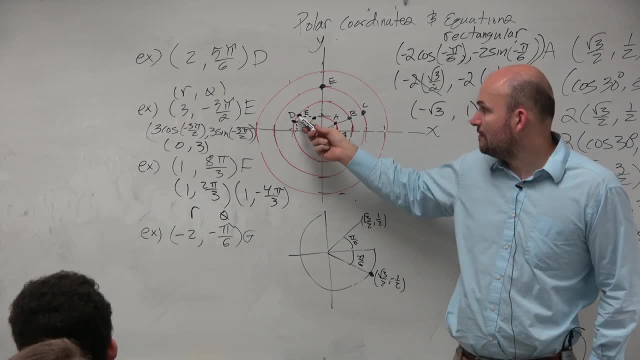 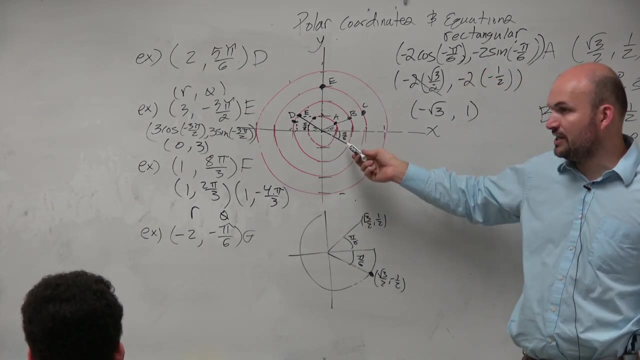 Well, first of all, to answer your question, to graph this correctly, that is the correct point. That's where it's graphed. But it kind of just gets confusing because if you graph negative pi over 6, that takes you over here. 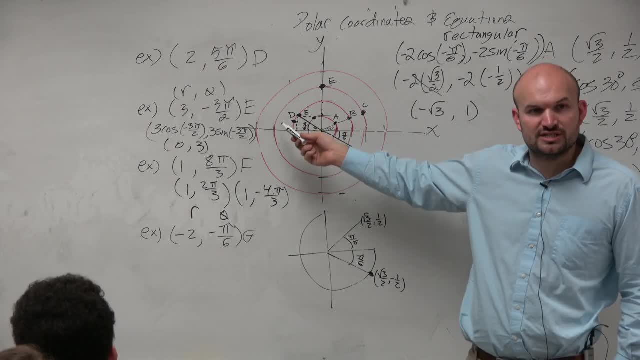 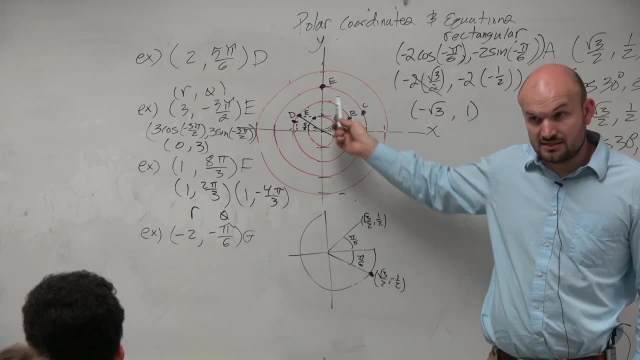 So what is this 2?? It looks like it's a reflection about the origin, doesn't it? It's reflected about the x-axis and then reflected about the y-axis. Yes, Yes, Doesn't it look like it's happening? No, 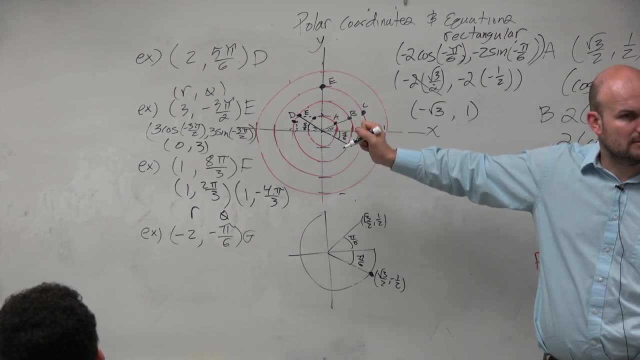 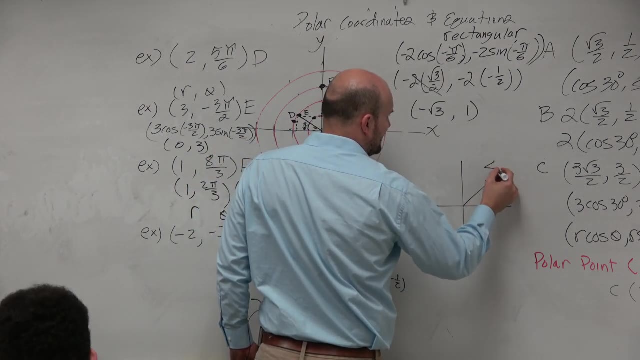 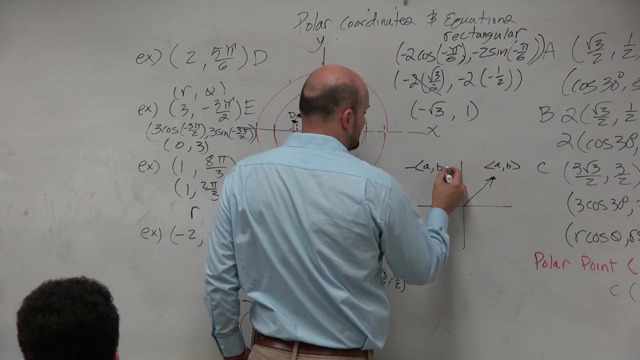 Okay, Have we experienced this before, Have we? What about in vectors? Remember we had a vector a- b. Does anybody remember what negative a b, What happened to that Reflected? You distribute that to both of them, right? 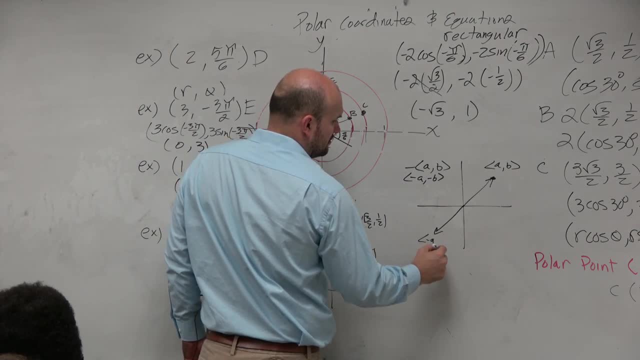 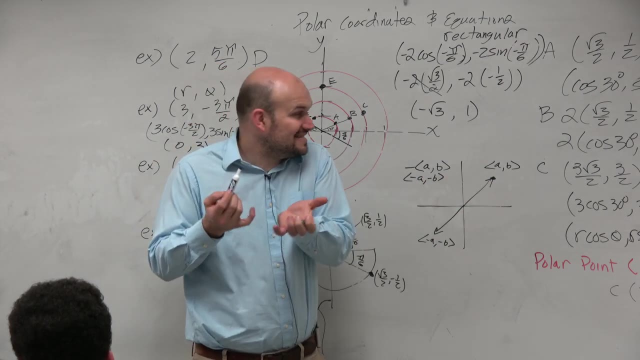 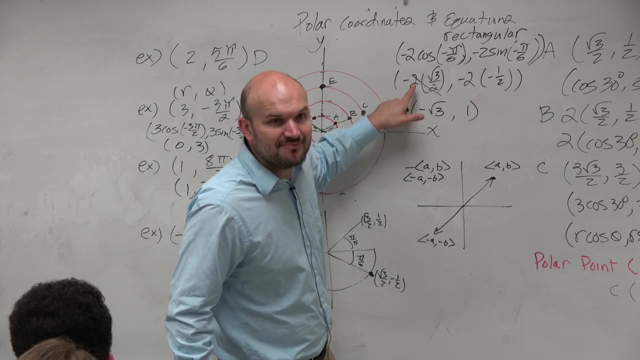 The scalar multiple. See how this got reflected about like the origin, And you guys got to think about that. That's exactly what this negative is. Because, guys, what did we just do with this r? The r multiplied by the x-coordinate and by the y-coordinate. 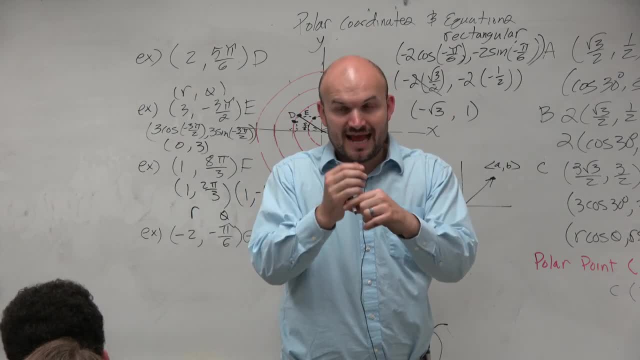 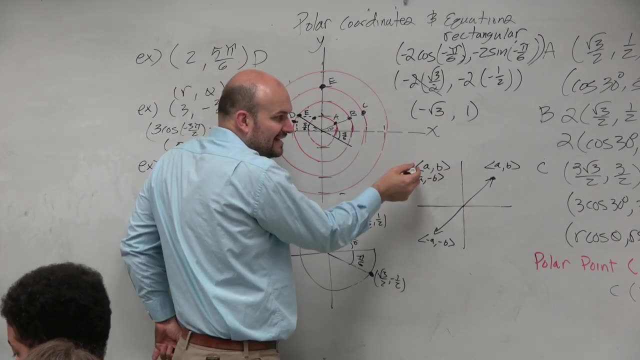 So when you have a negative radius, you're right, The radius is still r, but what the negative is doing is it's changing the direction. So this negative is technically a negative directional change. It's not a distance change, It's a directional change. 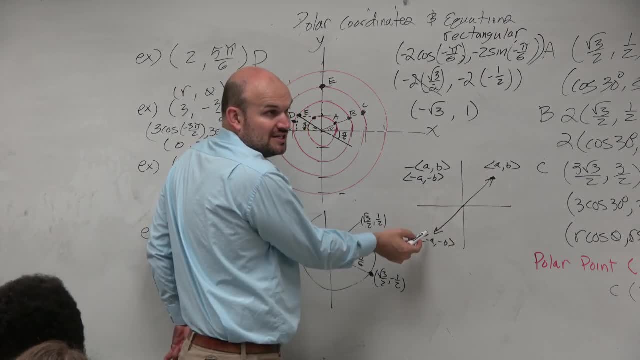 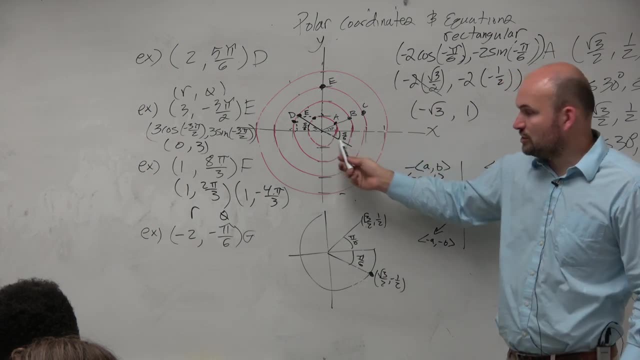 You guys see how the vector still has the same magnitude, Right, But what has changed? The direction, Right. So that's what happens. when you guys have this negative, You can basically find your original angle, and if you have a negative, you can just reflect it about the origin.